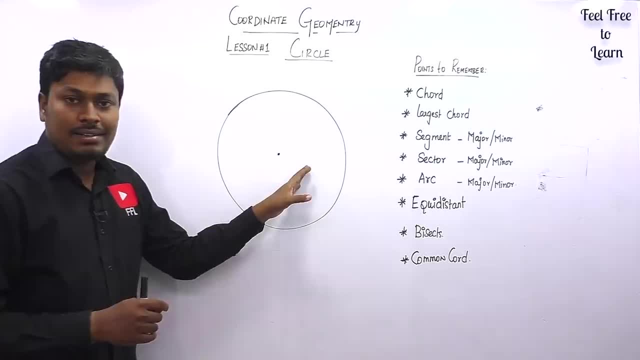 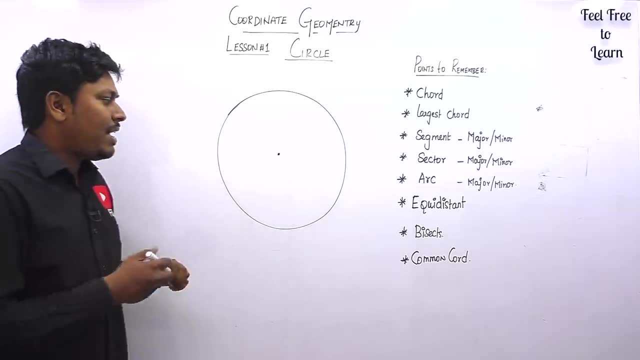 based on circles, And everyone knows if it is a circle. you know what is called as a center point, So this will be called it as center, Or otherwise we can call it as a fixed point. Got it? And every time we usually determine. 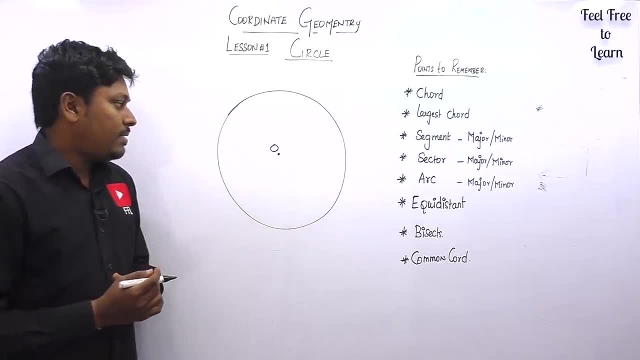 this as O, which determines the center of a circle, And next is a diameter and a radius. You guys have you know, this is called as a radius And this complete line is called as a diameter. Okay, so now in this video we are going to discuss about the chords. 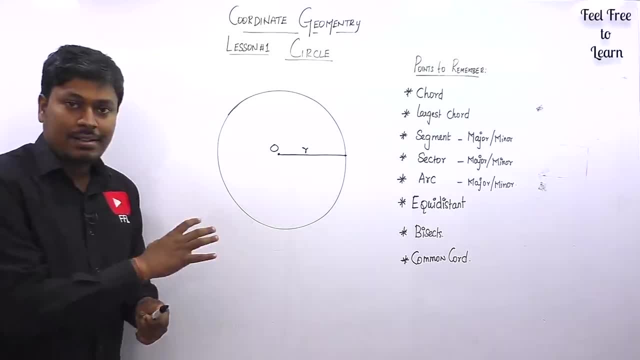 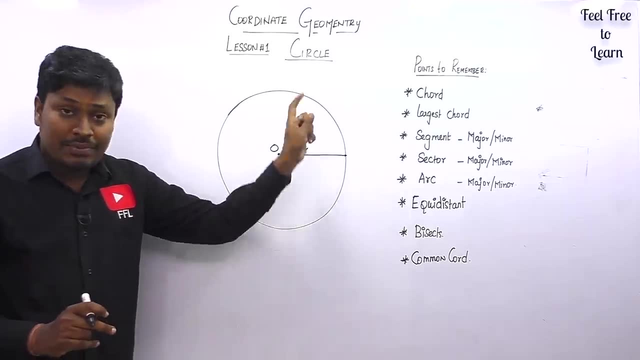 And next video, we are going to solve some question based on the concept chord chords, And in lesson number three we can learn about tangent and we can learn about the concept of chords. So first, these are the points that you guys have to remember before solving a question. 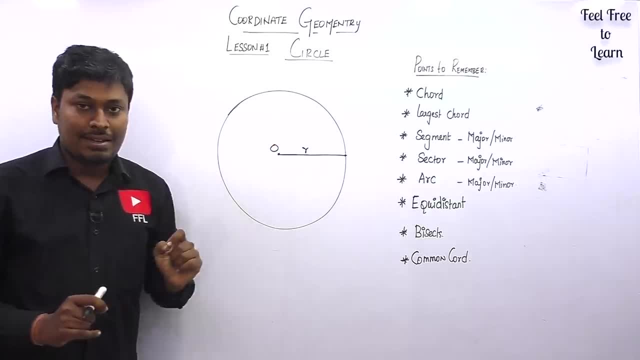 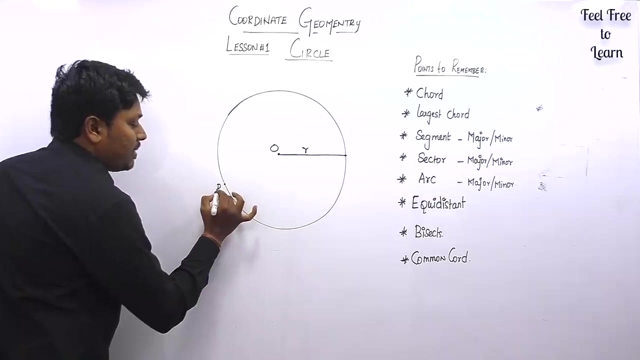 that is based on a chords. So first, what is a chord? So listen here. a line segment joining two points on a circle is called as a chord. Remember that. a line segment, right, joining two points on a circle. Let me take this is point number one, that is point P. 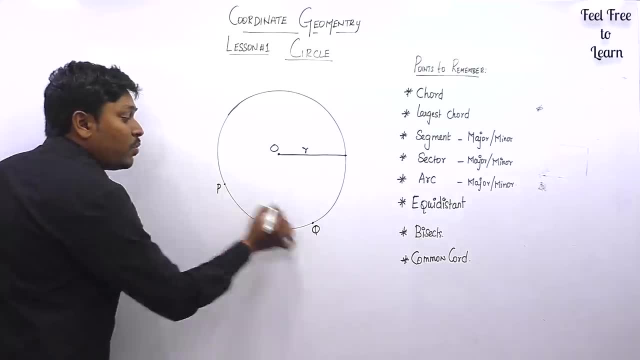 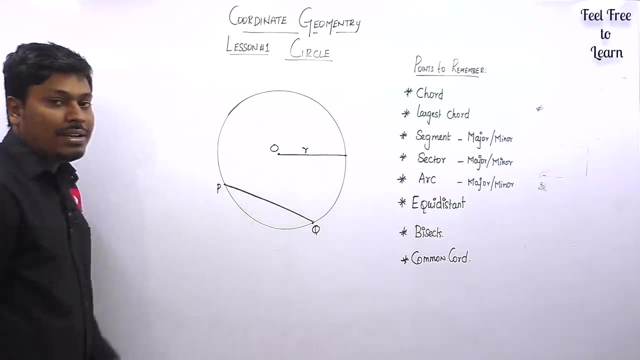 Got it And I am just taking this as point Q And I am going to join these two points or line segment which is called as a core. So this P and Q is called as a chord. A line segment that is connecting two points on a circle is called as a chord. We can drop around. 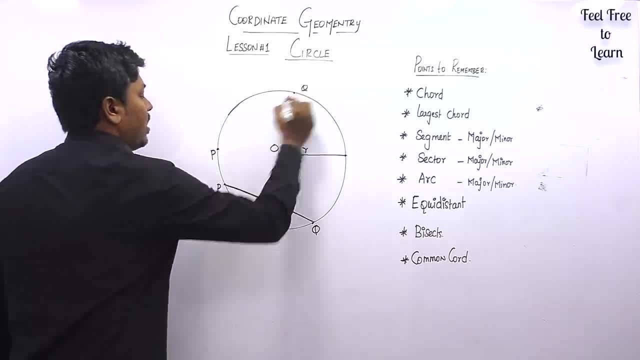 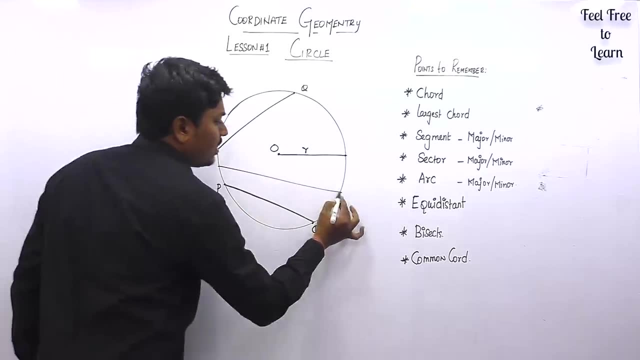 anywhere else. we can say point P here and point Q here and we can say it is one of the chord, because the line segment joining two points on a circle is called as a chord. that is, we can draw a chord here and we can say it is one of the chord. Similarly, we 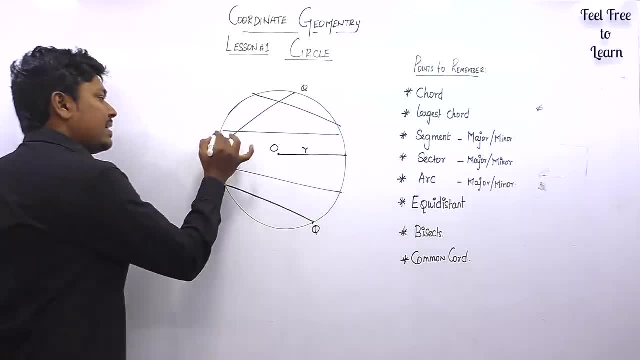 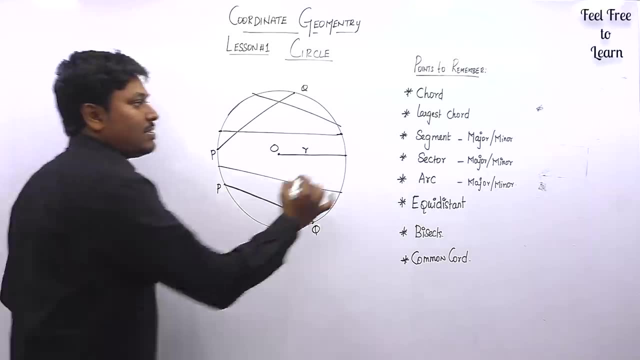 can draw another chord here. another chord here. remember that the meaning of quad is any two points that is connected by a line segment is called as a quad. So this is point number one that you guys have to remember. So point number two is the largest quad. So largest quad. I have an another name called diameter, So diameter can. 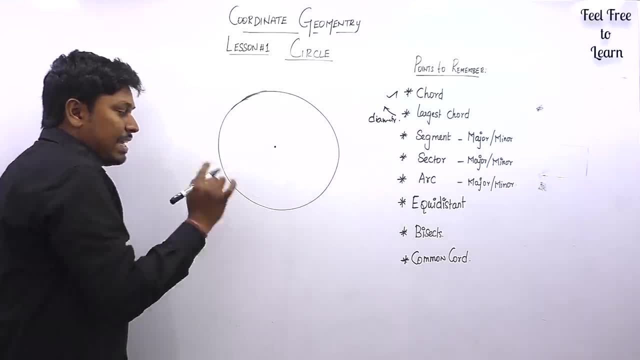 be also said as a largest quad. So remember that if a line segment that passes through the center point, then it is called as a diameter, or otherwise it can be called it as a largest quad. Friends got it. We usually say this as a diameter, right? We say this as a diameter of the circle, So 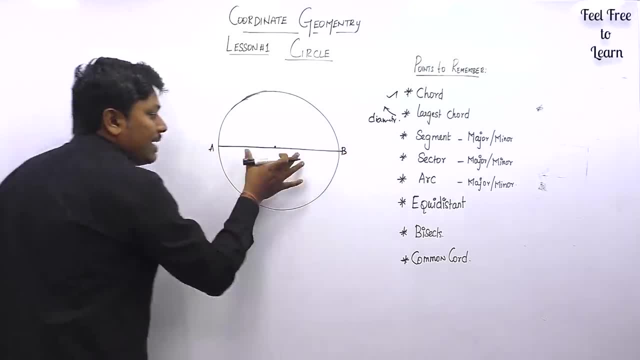 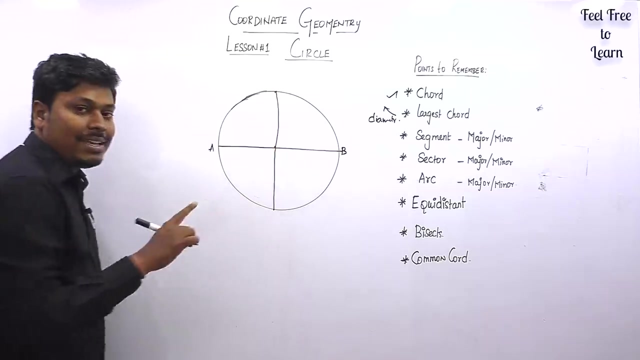 remember that this is point A and point B and the line segment that is connecting two points on a circle. we used to call it as a quad. So if a quad passes through the center point, right, we can say this also. If a quad passes through the center point, then we can say this as a largest quad, or. 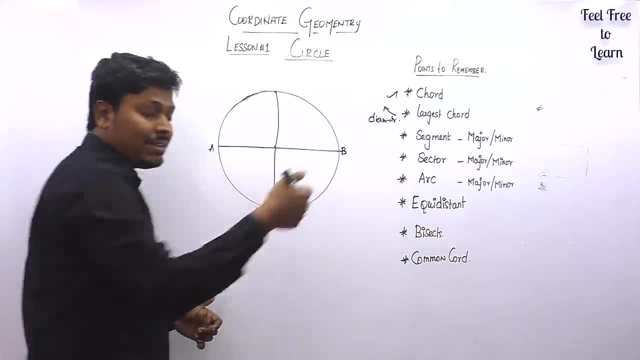 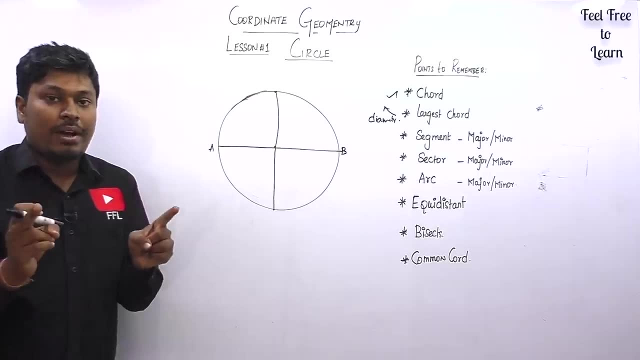 otherwise a diameter Got it So diameter. we have an another term, which is called as a largest quad. So quad. we know that. what is the meaning of quad? a line segment that is connecting two points is called as a quad. What is called as a largest quad? a line segment that passes through. 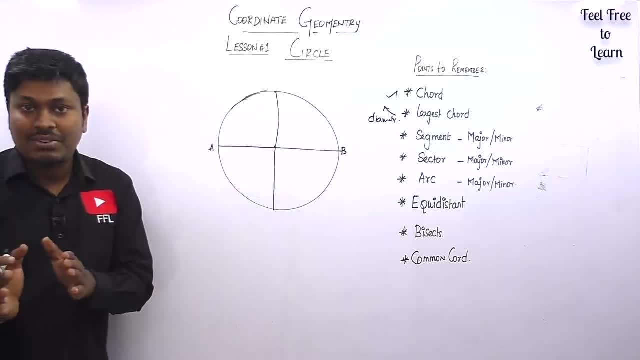 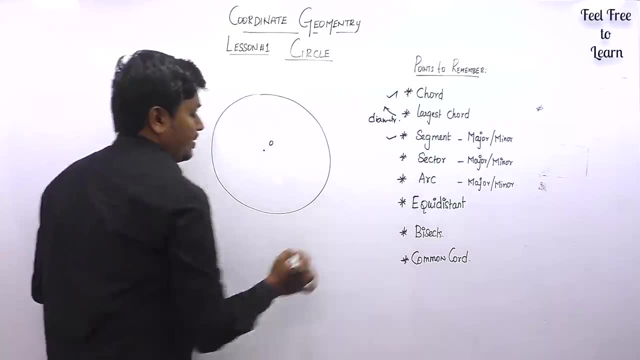 the center point of the circle. then it is called as a largest quad or otherwise. we can say the same largest quad as a diameter. Note number three. So note number three is a segment. So listen, here I am just going to draw any quad Here. let me assume this is point A and point B. 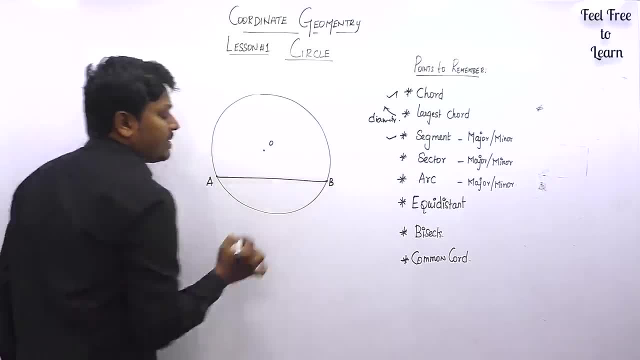 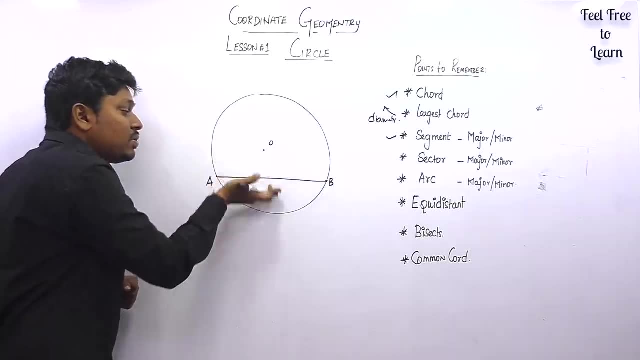 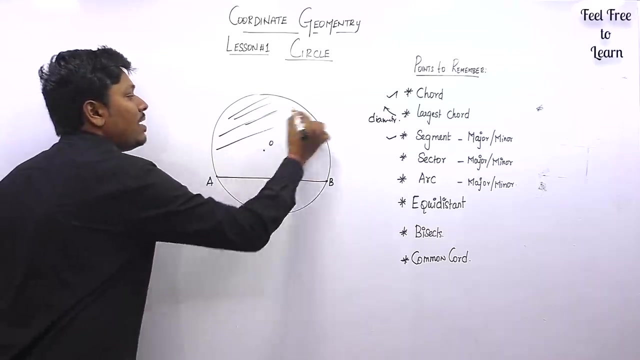 and we can connect these two points by a segment so we can say A and B will be a chord. So this line segment divides the circle into two segments. right, got it, friends. So this line divides the circle into two segments. that is, this segment is called as a major segment and this is. 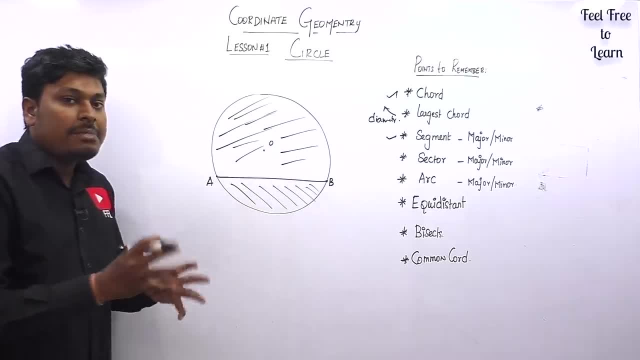 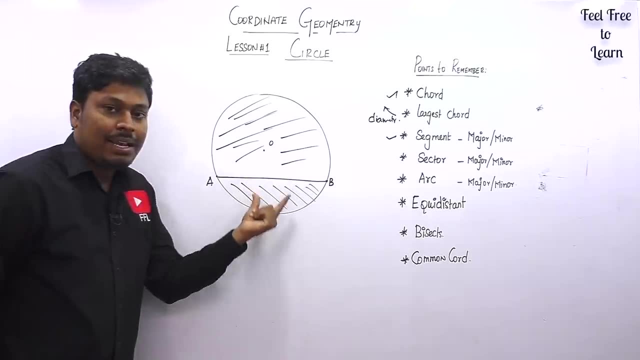 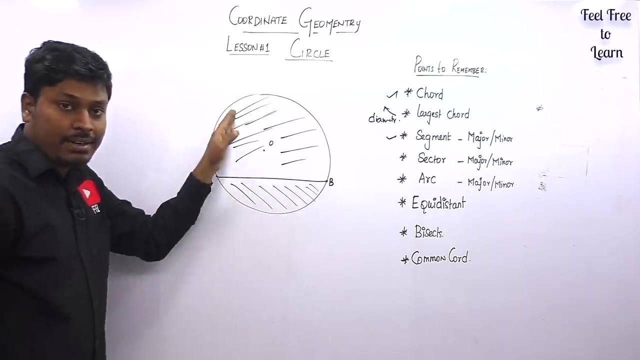 called as a minor segment. So minor is nothing but a minimum part. major will be a maximum part, So a chord that divides a circle into a major segment and a minor segment. So remember that the word major determines the maximum part, because this chord divides a maximum part here and a minimum part at the below. So we can say: 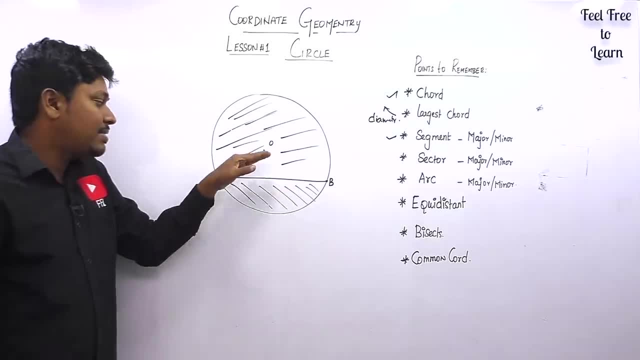 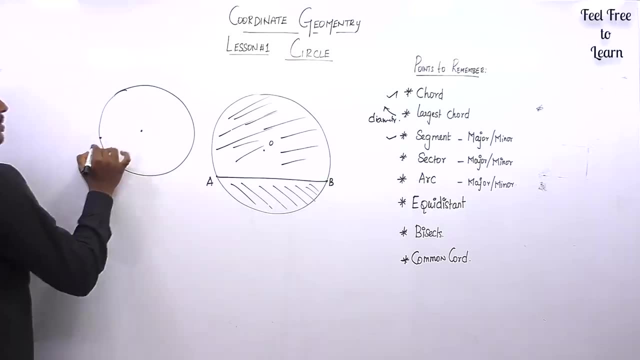 this will be the minor part. that is minor segment and this is called as a major segment, right, got it? So, in case, think that I am drawing a chord here, so A here and B here, So A and B be the chord, So we can say which is the major segment. 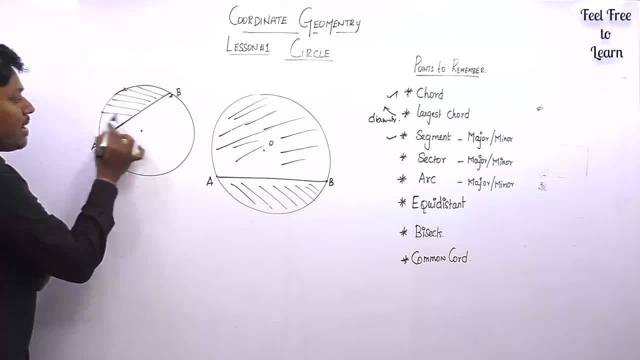 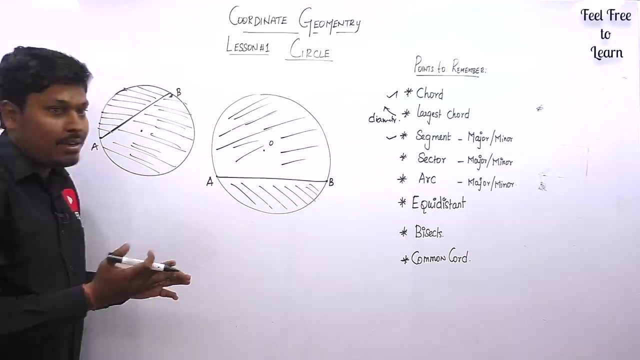 and the minor segment. So this will be the minor segment minimum area and this will be the major segment maximum area. So got it, friends. If a chord passes through the diameter, that is, if a chord passes through the center, then we can say we won't have a major and minor segment. So 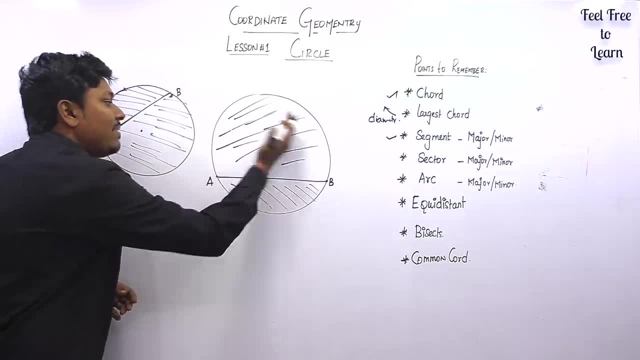 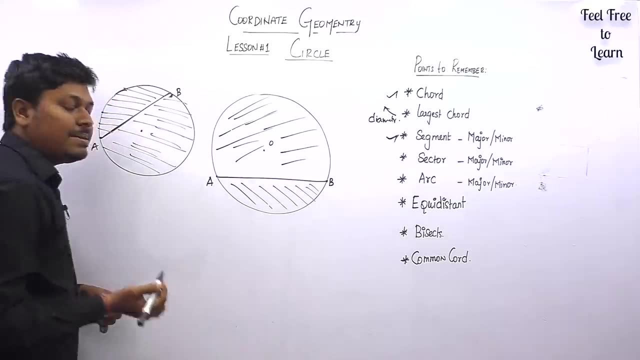 if a chord that passes through the center of the circle, then it divides the circle into two semicircles, got it? So this is the thing that we call it as a major segment and a minor segment, And next is a sector. So sector is nothing. 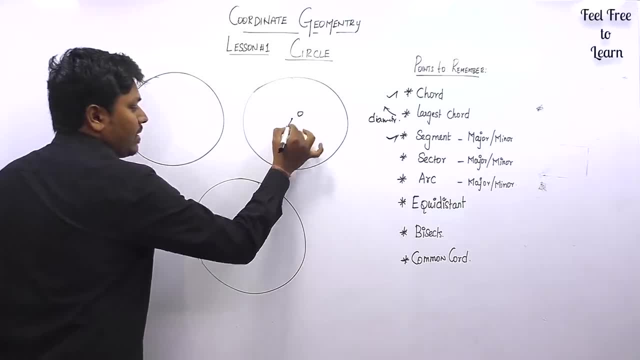 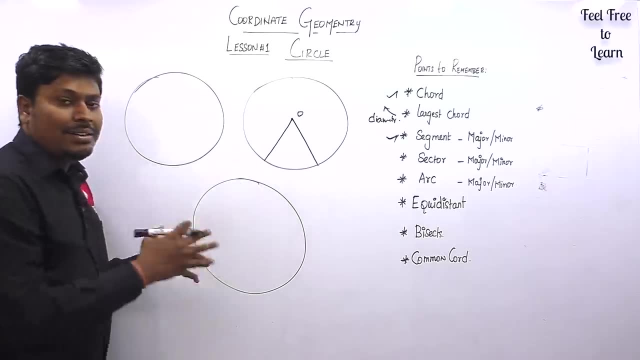 but, for example, if we keep this as center point O and we can say, if you can easily say this will be the one sector, right, We always know that, right, if, if it is a circle, we can split into 4, 6,, 4 sectors, 6 sectors, 8 sectors easily. So 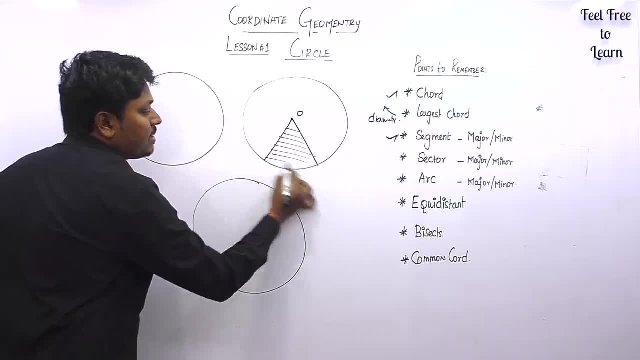 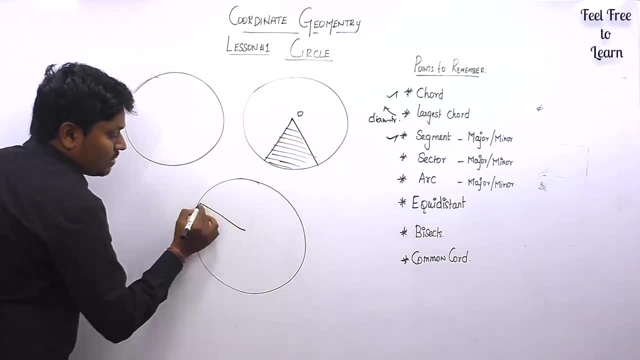 according to this part, we can say: this will be one sector which is a minor sector, right, a small part, and the remaining will be the major sector. got it, friends. Similarly, we can draw like, draw like this. Once you draw like this, then we can say it will be the. 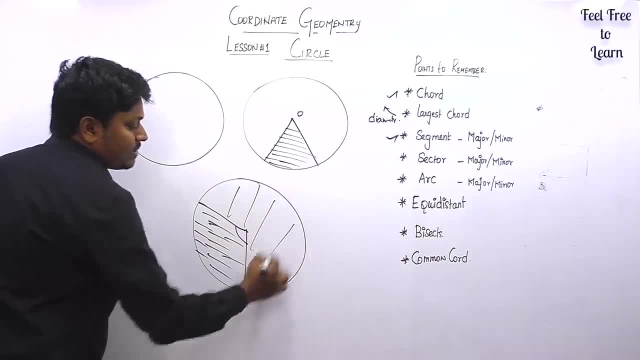 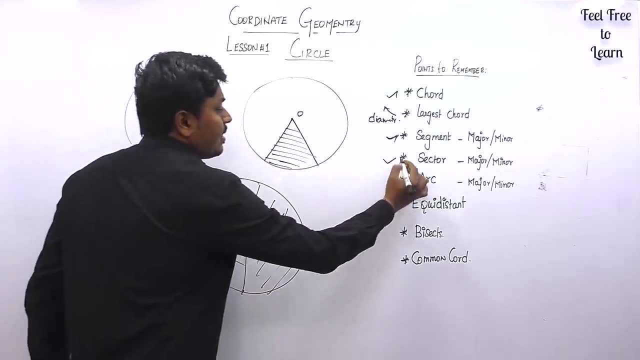 minor sector and this will be the major sector: a maximum part which is called as a major, and minimum part which is called as a minor. So this is called as a major sector and a minor sector. So next is a major arc and a minor arc. 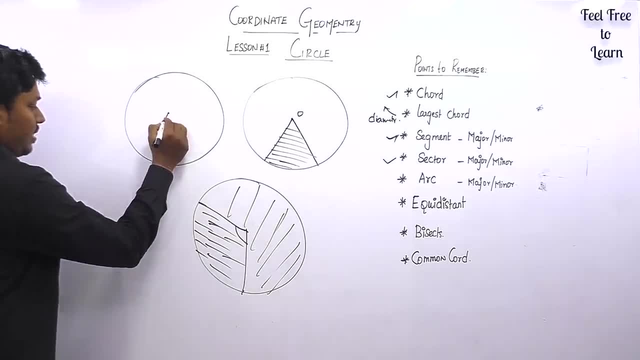 So the same word, for example. see here, friends- most important, let me fix it- think that this is an angle, something is like 30 degree here, and this will be the center point and we can mention this as A and B. So the meaning of major and the minor arc is from A to B. it is just a small arc, right? 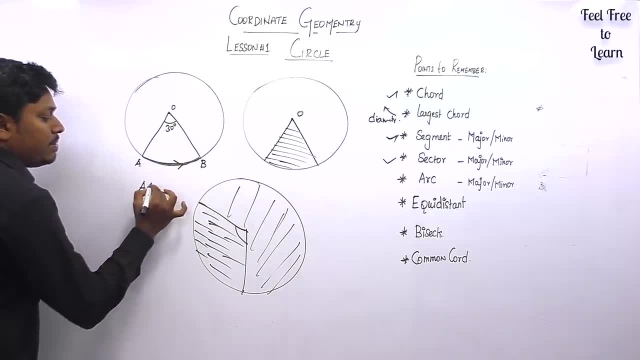 A to B will be a small arc. So we can say A and B will be the minor arc, But when we talk about B to A will be the major arc. friends got it. If we draw a sector like this, then we can say this will be the minor arc because small. 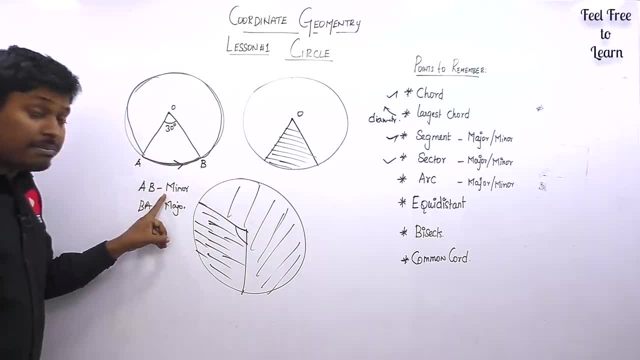 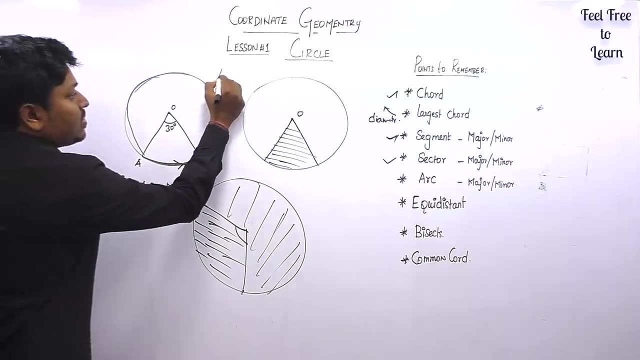 portion. we used to call it as minor. So A to B will be the minor, But B to A will be the major arc. Sometimes the same thing can be also written as they usually write, like this: AB at the top. they used to determine like a small symbol. 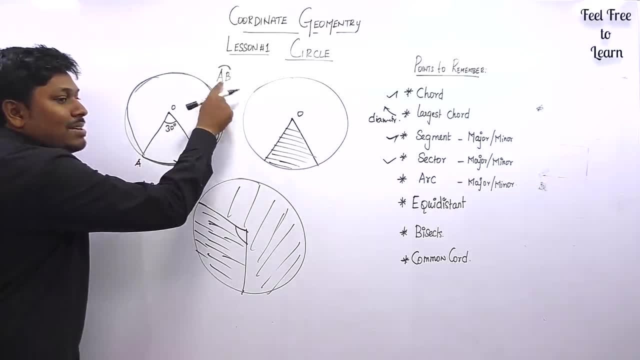 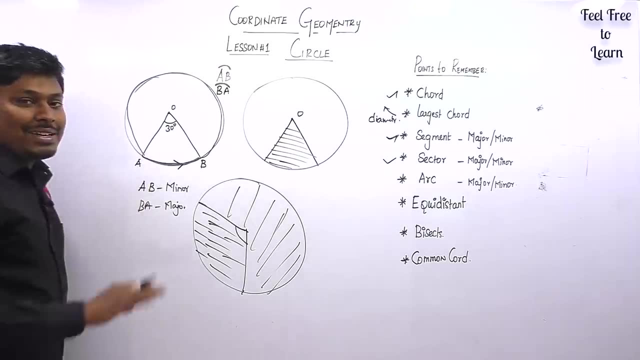 So which determines an arc right, A to B will be the minor arc and B to A will be the major arc. So this determines arc right. So similar to the vector right. usually they in the vector topic. we will be writing like this: A vector, B vector. 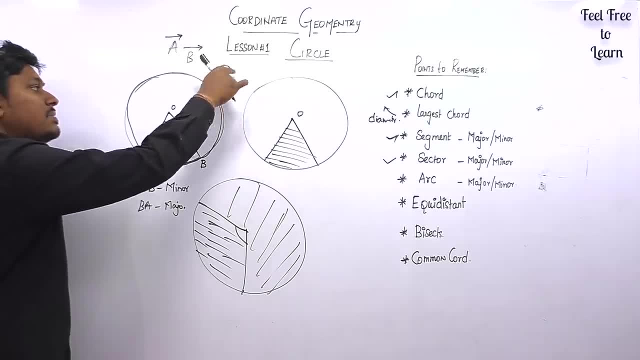 So similarly in the geometry. So in the geometry topic, if they determine like this, which is called as a arc, So A to B, a small part, which is called as a minor arc, and B to A will be the major arc, got it friends. So this is called as minor and the major arc. 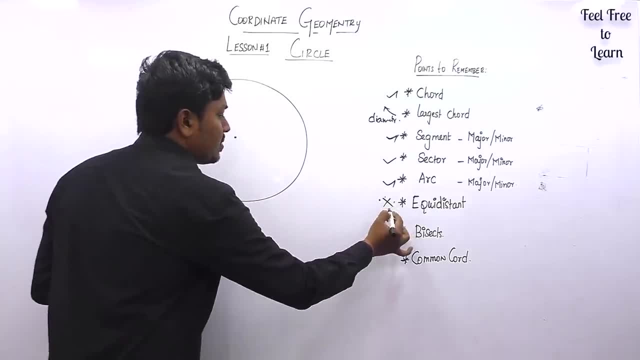 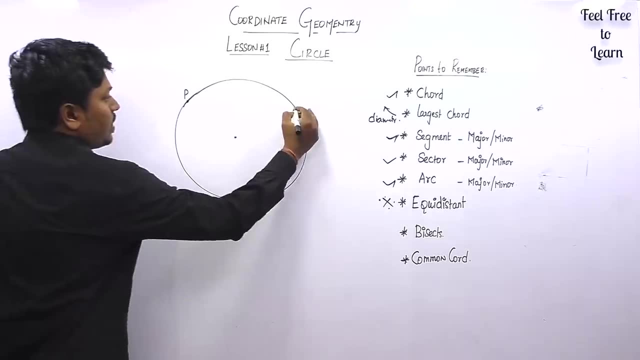 And next is the equidistant. So equidistant will is most important to solve many question in the topic circle. So remember that if there are two chords- let me assume this is chord 1- P and Q here, And similarly we can assume B and Q here. 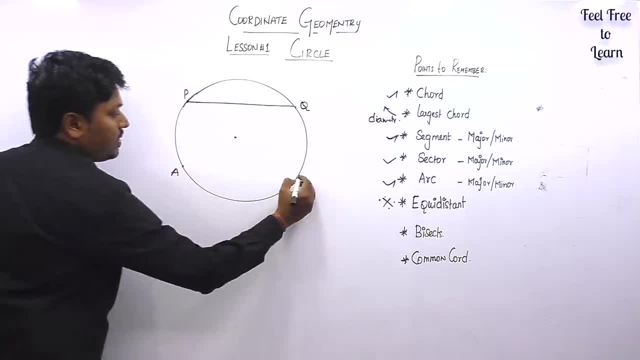 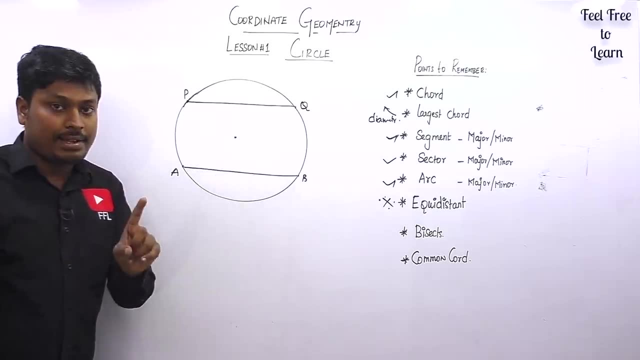 So this is the major arc. Similarly we can assume on another chord, A and B. here Listen carefully, friends. If two chords of equal length, if two chords, that is, P and Q and A and B, are equal in length, then the distance between both the chords from the center will also be same. that is. 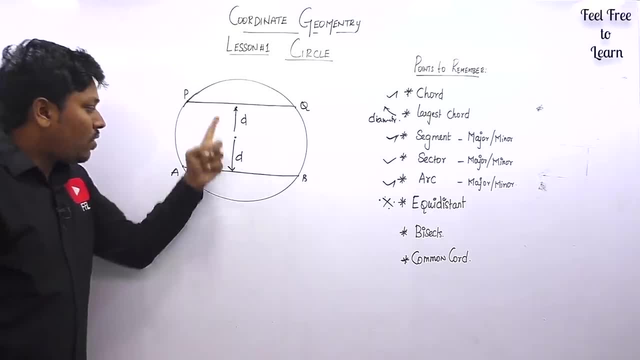 called as equidistant. So friends got it. If two chords of same length, then the distance between both the chords will also be same from the center. So this is called as an equidistant concept because a circle, right if one, two if both. 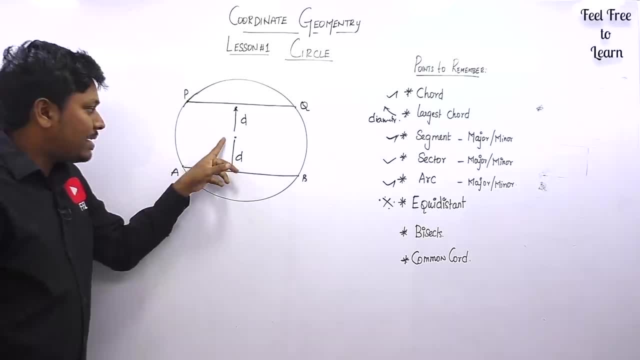 the chords are same in length, then we can surely say from the center point, both the chords will be at the same distance, So which we used to call it as a equidistant. that is it right. So next is a bisect. So now we have learnt, it is most important because we will be solving many question only. 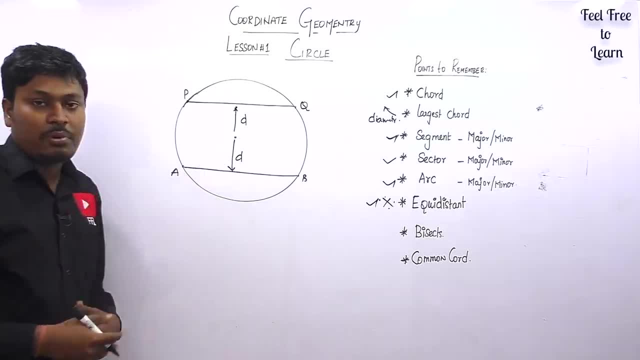 based on the equidistant concept. So remember, equidistant is important and next is bisect. So bisect is nothing, but, For example, think that P and Q is a chord right. So from the center point, if I draw a perpendicular line to the chord, it always bisects. 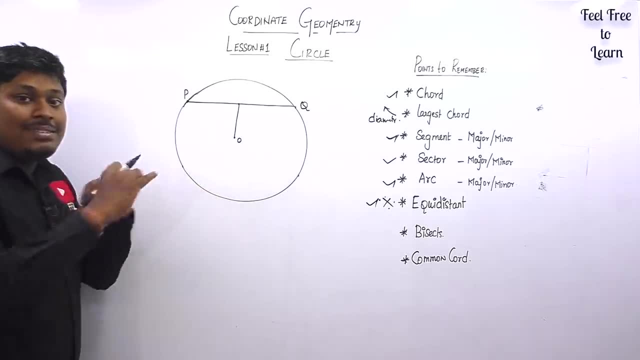 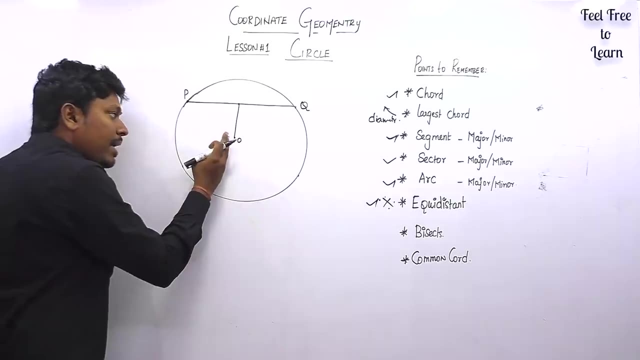 The meaning of bisect is it splits the line right. It splits the line segment into two equal of See. here we know that this is a chord From the center point. I am drawing a perpendicular line to the chord. it bisects the chord at. 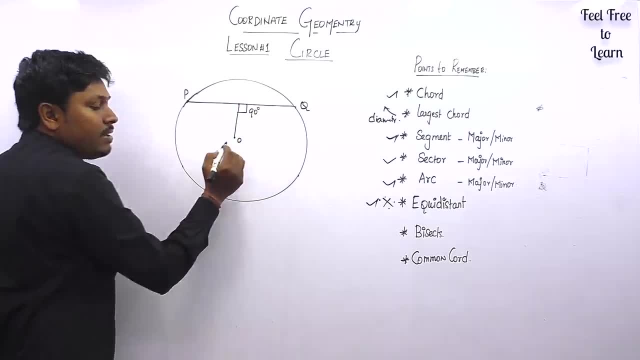 equal distance. Can you see? it is 90 degree. definitely it will be 90 degree and because of this perpendicular line where this chord is divided into two equal of. So this will be one equal of and this will be another equal of, For example. any point, let me take this as P and Q. 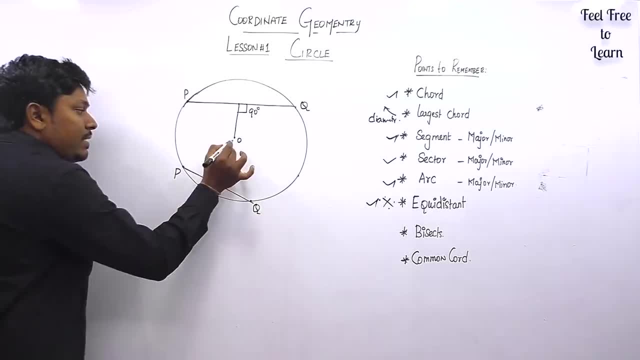 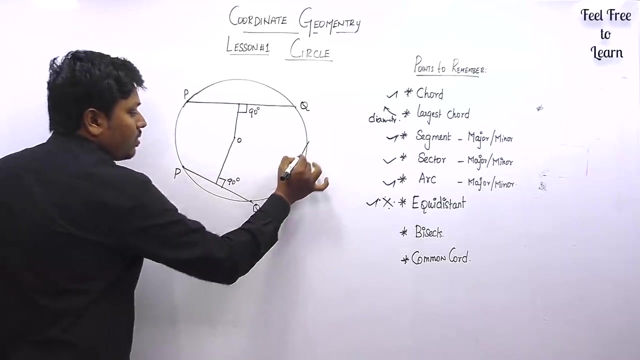 So P and Q. we can take another chord here. if I draw a perpendicular line from this center point to this chord, definitely this line will bisect The meaning of bisect. it splits the line into two equal of. So we can say this will be 90 degree. friends got it, even if you draw a chord here again. 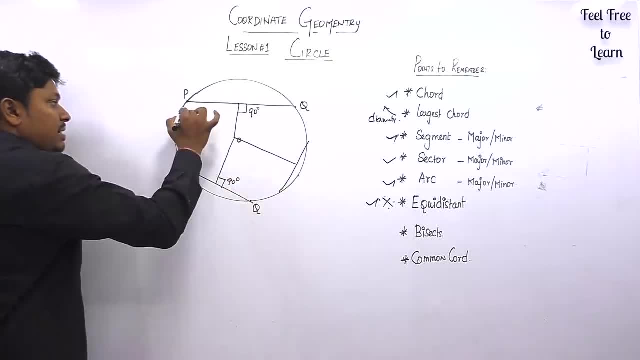 if you draw A perpendicular line from the center point, it bisects. Similarly, if you draw a chord like this from the center point, if you draw a perpendicular line, again it bisects the chord. that is it right? So the meaning of bisect is it splits the line into two equal of. 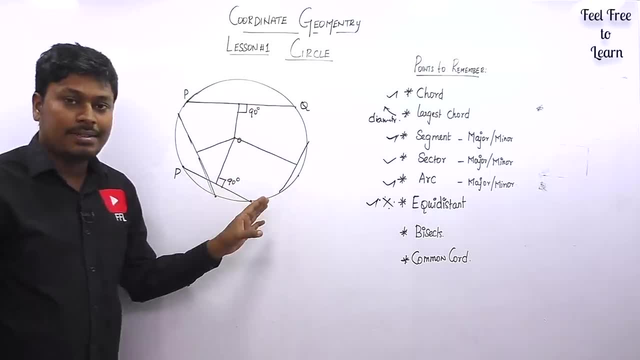 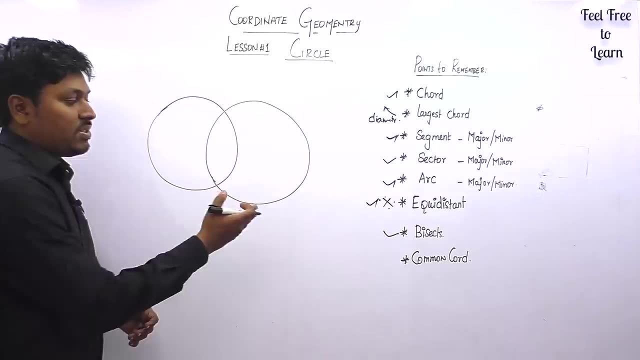 So remember that if you draw a chord anywhere else in the circle and if you draw a perpendicular line from the center point, definitely that line will be bisects the chord. So the last is the common chord. So common chord, Let me assume. 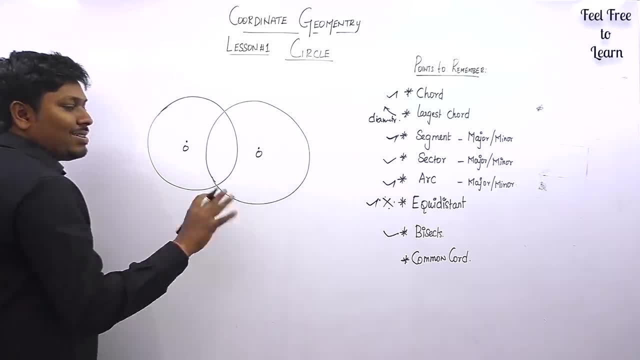 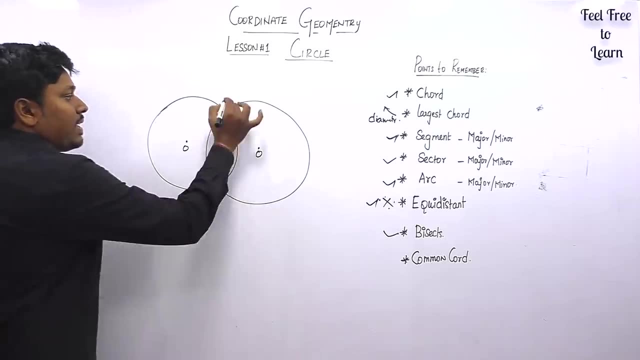 A common chord is nothing but a chord that should be common for both the circles. So we can draw a line like this by connecting two points So we can say this as A and B, So we can say A and B will be the common chord for both. 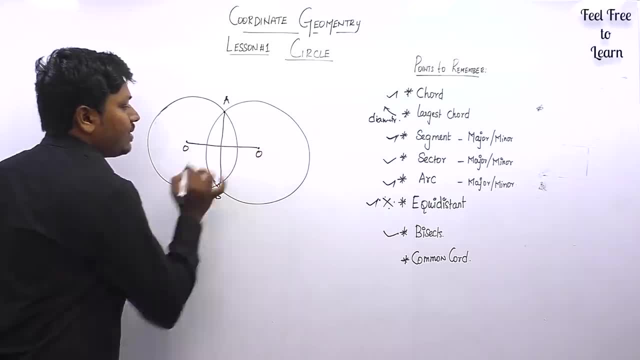 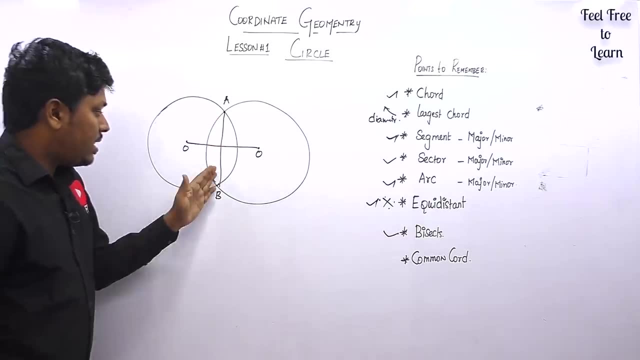 the circles And this chord will be perpendicular to the line joining the center. This will be the line joining the center of two circles, which is perpendicular to that chord Chord difference. So remember that A and B will be the common chord And also this A and B. 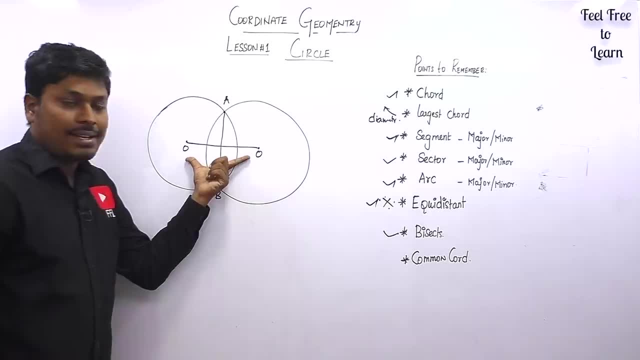 is the line that is perpendicular to the line joining both the centers. that's it, right? this is called as a common cot, So it's completely. there are many properties, there are many theorems, but that is not needed for the competitive exams, right, if you are going for a competitive exam. 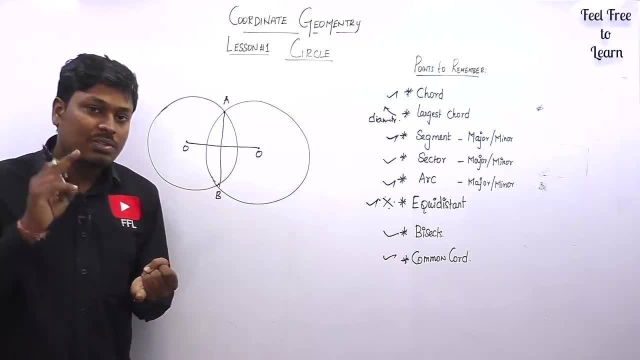 these are the segments are most important. So first you guys have to know what is called as a cot, what is called a line segment that is joining a two points on a circle is called as a cot, and what is called as a largest cot. if a same line segment, it crosses through the center point, then 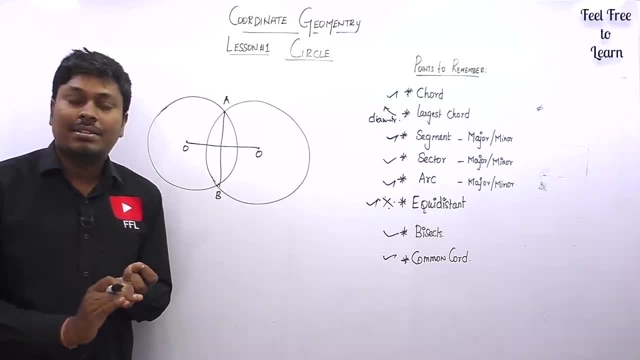 it is called as a largest cot, So we can also say the largest cot as a diameter, unless next is a segment. So once we draw a cot anywhere else on the circle it divides the circle into two half. that is, one will be the major segment and another will be the minor segment. If a cot that passes